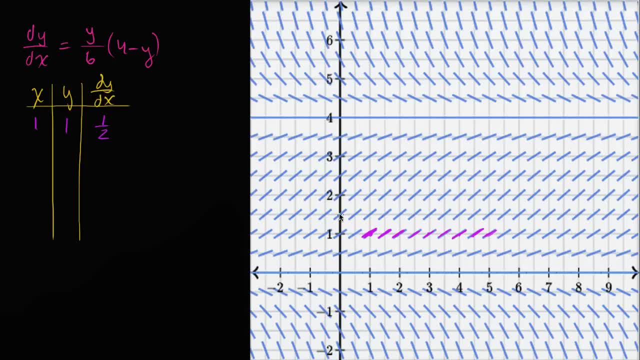 just to feel a little bit better about it. And then we will use the slope field to actually visualize some solutions. So let's say I don't know. let's do an interesting point. Let's say we have this point Actually. no, that's at a half point. 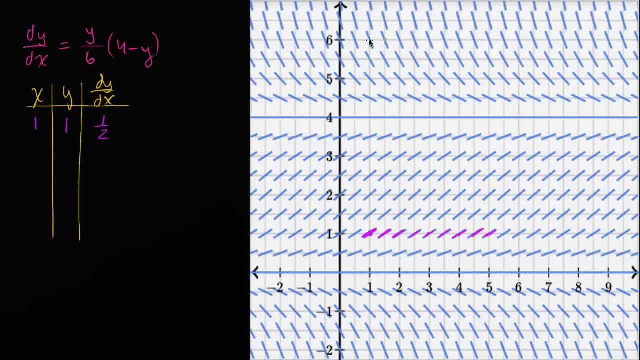 Let's say we have this, let's see I want to do. let's say we do this point right over here. So that's x is equal to one and y is equal to six, And we see the way the differential equation is defined. 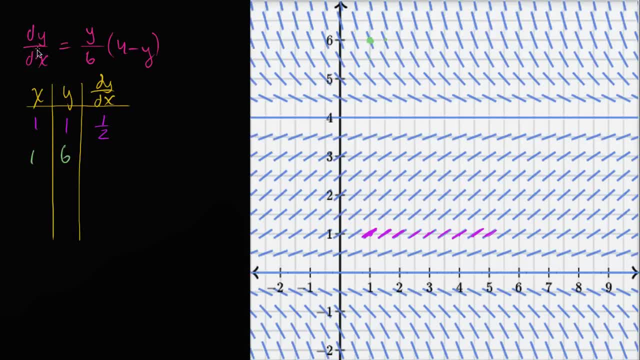 It doesn't matter what our x is, It's really dependent on the y that's going to drive the slope. But we have six over six, which is one times four minus six, which is negative two. So it's negative two. 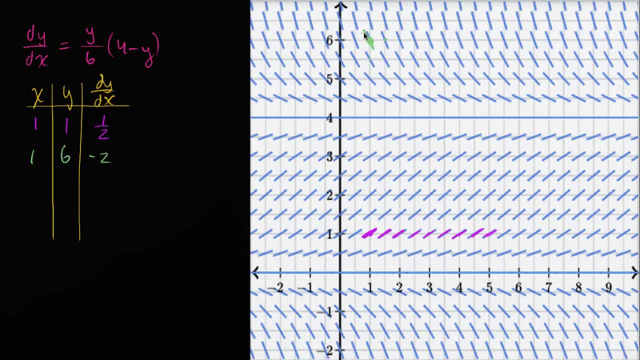 So we should have a slope of negative two And it looks like that's what they depicted. So as long as y is six, we should have a slope of negative two, Have a slope of negative two And you see that in the slope field. 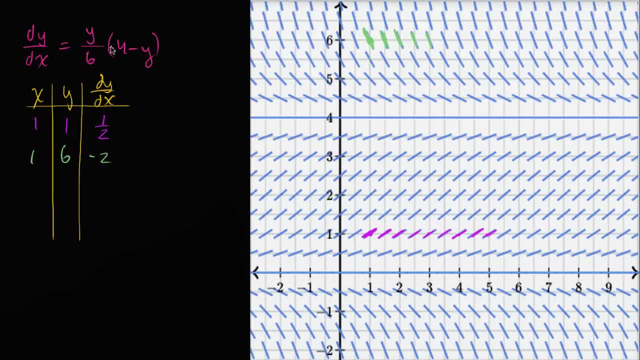 So hopefully you feel pretty good that this is the slope field for this differential equation. If you don't, I encourage you to keep verifying these points here. But now let's actually use this slope field. Let's actually use this to visualize solutions to this differential equation. 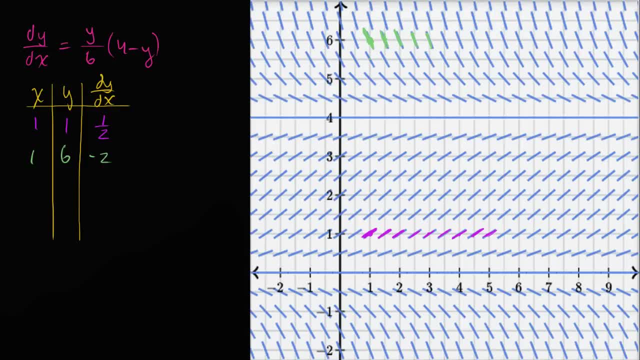 based on points that the solution might go through. So let's say that we have a solution that goes through this point right over here. So what is that solution likely to look like? And once again, this is going to be a rough approximation. 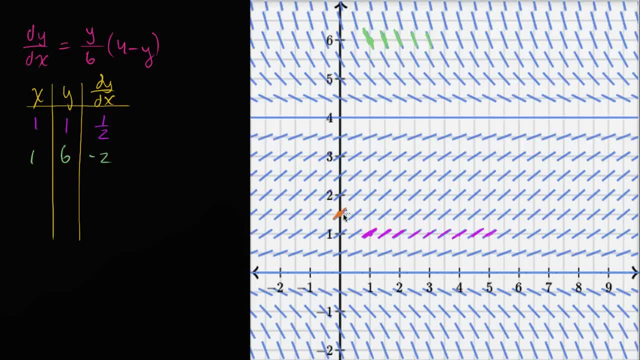 Well, right at that point it's going to have a slope. just as the slope field shows And as our y increases, it looks like our slope. it looks like our slope. so at this point I should be actually. let me undo that. 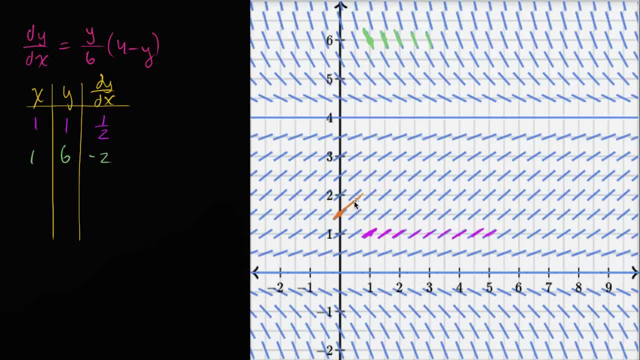 So this: if I keep going up at this point, when y is equal to two, I should be parallel to all of these segments on the slope field at y is equal to two And then it looks like the slope starts to decrease as we approach. y is equal to four. 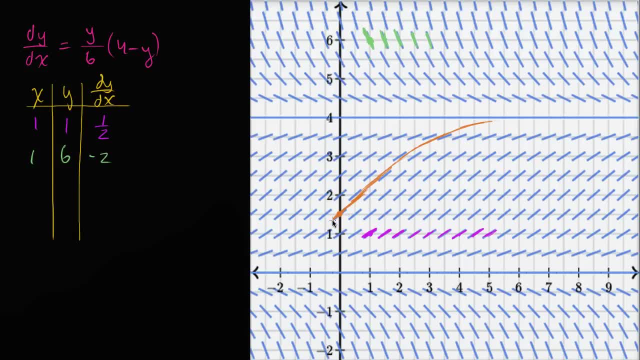 And so if I had a solution that went through this point, my guess is that it would look something. and then now the slope decreases again as we approach. y is equal to zero, And of course we see that, because if, when y equals zero, this whole thing is zero. 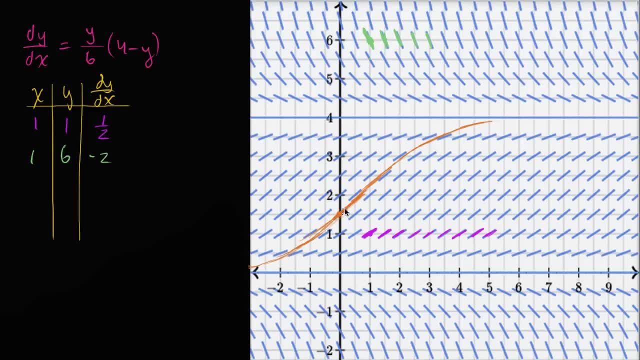 so our derivative's going to be zero, So a reasonable solution might look something like this. So this gives us a clue. Well, look, if a solution goes through this point, this right over here might- this might actually be what it looks like. 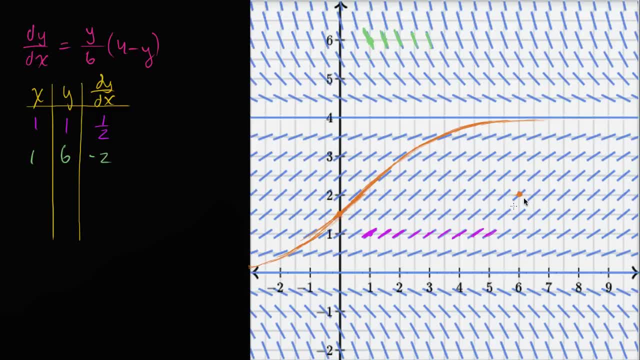 But what if it goes through? I don't know what. if it goes through this point right over here? Well then it might look like. it might look like this, by the same exact logic. So it might look like this. So, just like that, we're starting to get a sense. 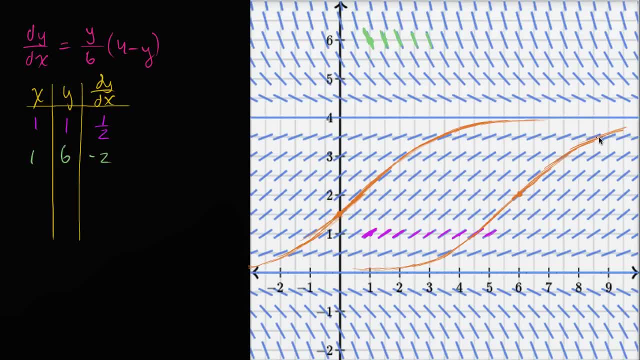 We don't know the actual solution for this differential equation, but we're starting to get a sense of what type of functions. what type of functions are the class of functions that might satisfy the differential equation. But what's interesting about this slope field is it looks like there's some you know. 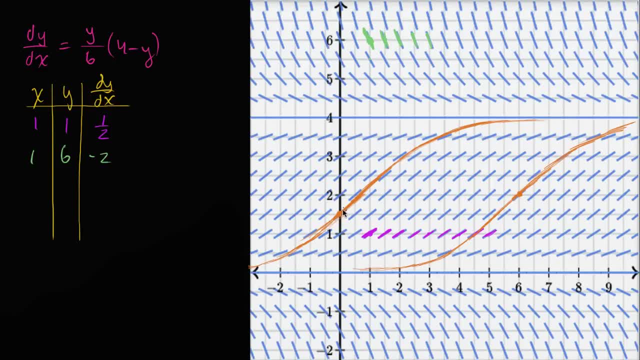 there's some interesting stuff you know if we have. if our solution includes points between where the y values between zero and four, it looks like we're gonna have solutions like this, but what if we had y values that were larger than that? 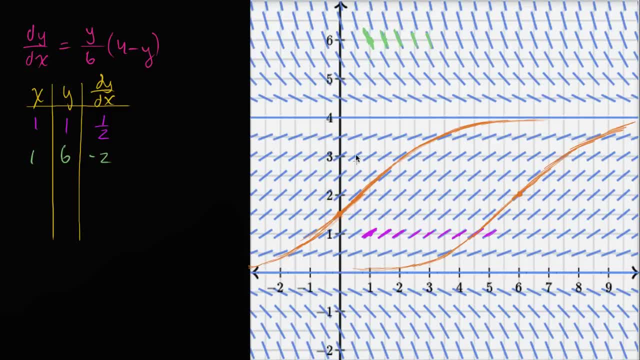 or that were less than that, or exactly, exactly zero or four. So, for example, what if we had a solution that went through this point right over here? Well, at that point right over here, the slope field tells us that our slope is zero. 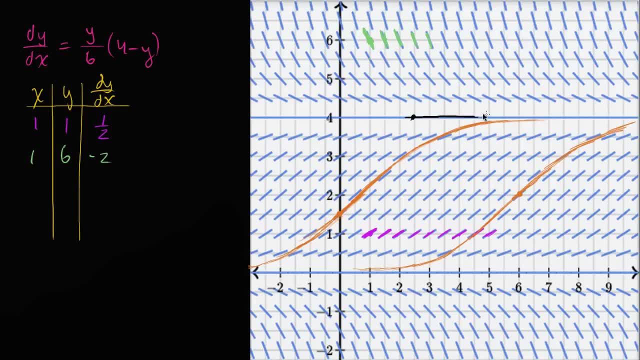 so our y value's not going to change. and as long as our y value doesn't change, our y value's gonna stay at four. so our slope is going to stay zero. so we actually already found this is actually a solution to the differential equation. 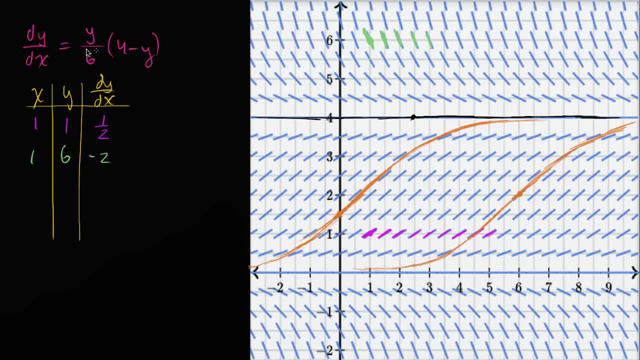 it's y is equal to four is a solution to this differential equation. So y is equal to four, y is equal to four and you can verify that that is a solution. When y is equal to four, this right hand side is going to be. 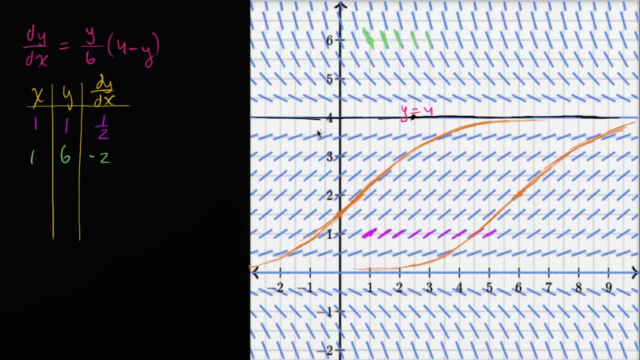 zero and the derivative is zero. for y is equal to four. so that is a solution to the differential equation. And the same thing for y is equal to zero. That is also a solution to the differential equation. Now what if we included points? 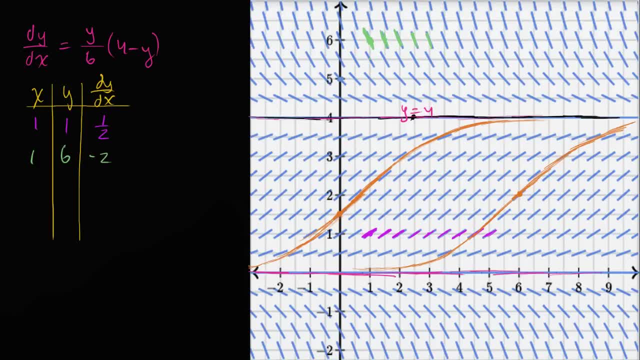 what if we included this point up here and actually let me do it in a different color so that you could see it? Let's say, our solution included that point. Well then it might look something. it might look something like this: